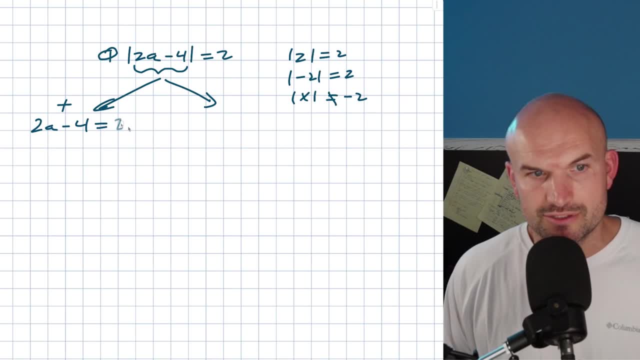 remove the absolute values and you're going to say, well, I know, this can be equal to a positive 2.. And then, for the negative case, you say, well, this could also equal to a negative 2, right, Because the absolute value of negative 2 is still 2.. So what I'll do is I'll just now take the 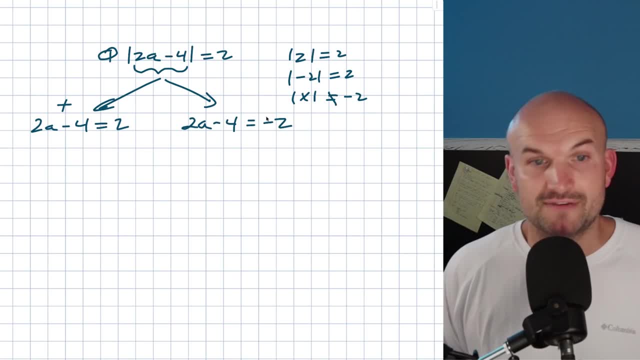 again remove the absolute value symbols, and then I'll just set it equal to a negative 2.. Now you can see that I have a linear equation, though, that I can simply now just go ahead and solve. So I'll just go ahead and use my inverse operations here, and I get a 2a. 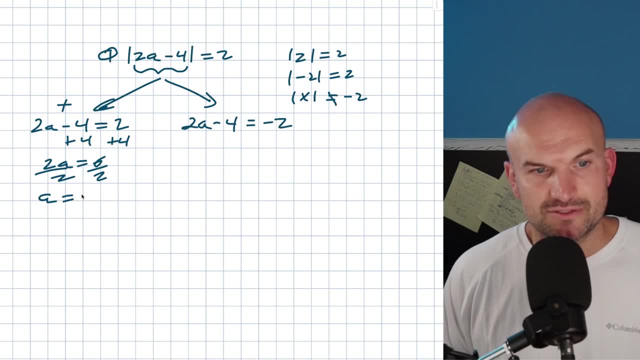 is equal to a 6, divide by 2,. divide by 2,: a is equal to a 3.. And then over here I could add a 4 to both sides and I can get a. 2a is equal to a positive 2, divide by 2,. divide by 2,. 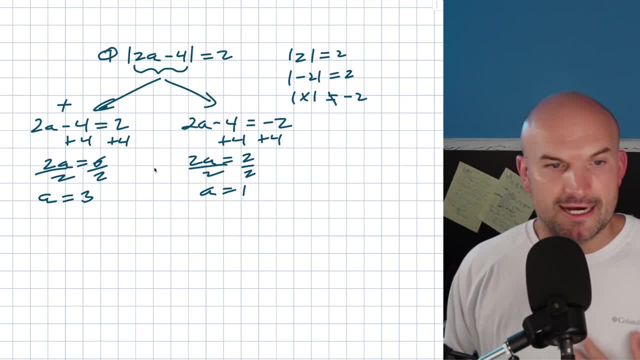 a is equal to a 1.. Now it's always important to kind of like check your answer to make sure that you're not dealing with extraneous solutions And to review like extraneous solutions are just going to be solutions that make an equation true, but that do not satisfy the original. 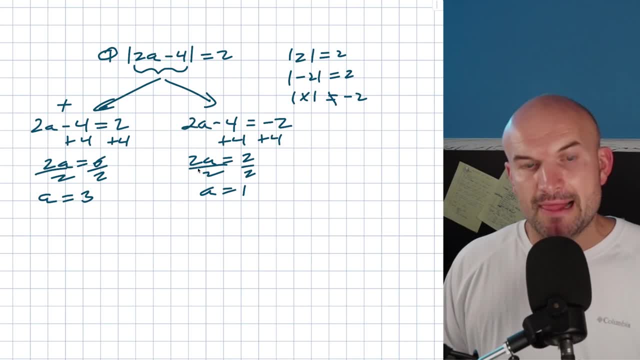 equation. So you could solve for these three equations, You could get two answers and they are going to satisfy these two equations, but they don't necessarily always go ahead and satisfy our original equation. However, in this case you can see like as long as you plug these back in. 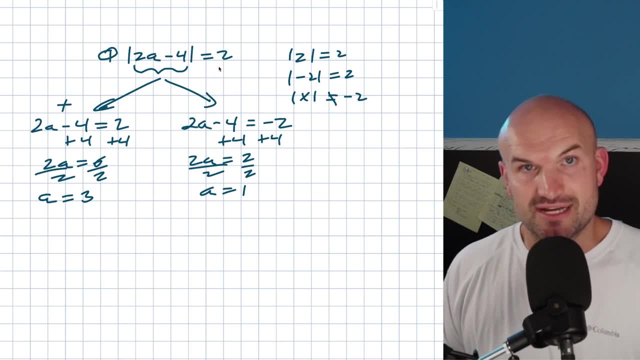 as long as you're getting back a 2 or a negative 2, it's going to satisfy the equation on the other side, right? So I'm just going to do a little bit of mental math. When I plug 3 back in, that gives me a 2.. When I plug a 1 back in there, that's going to give me a negative 2.. 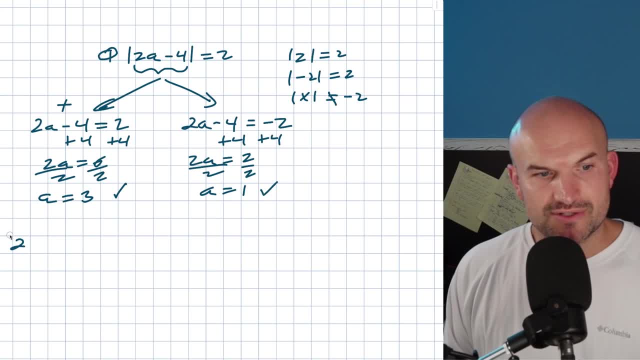 So therefore, these are both satisfied here, All right. So now let's go and take a look at another example. What if we have some things outside of our absolute value? For instance, negative 2 times w plus 9 is equal to a negative 2.. Now one problem that happens with students a. 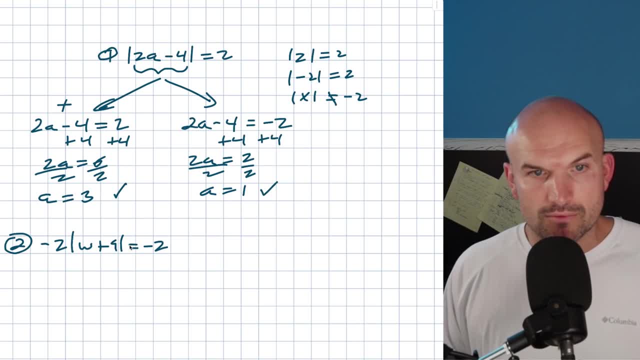 lot of times on an example like this is: they all see, oh like, oh crap, Like we have it equal to a negative. 2. Like there's no solution. Yeah, yeah, yeah, But the absolute value is not isolated. 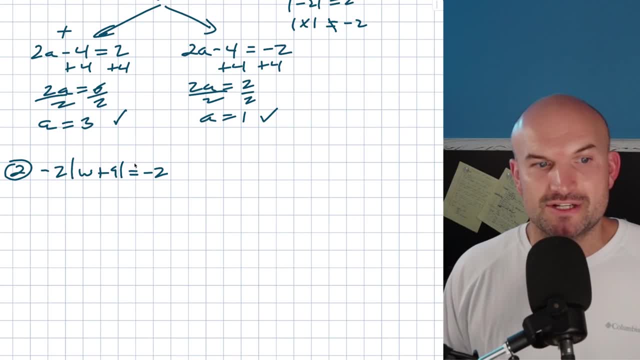 right. So the first thing you always want to do when solving an absolute value equation is go ahead and isolate this absolute value sign. okay, So when we isolate the absolute value, what we're going to do is basically use my inverse operations to undo whatever is being. 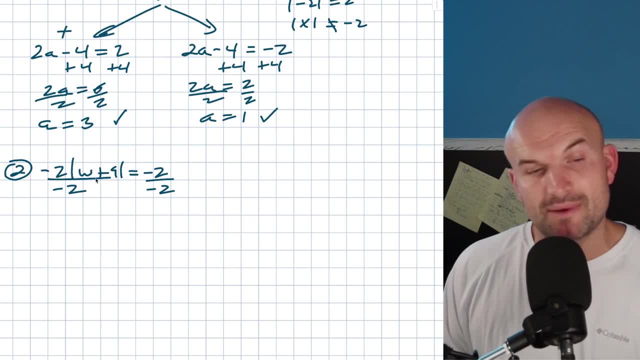 applied to the absolute value. So in this case you can see that the negative 2 is multiplied by the absolute value. So I'm going to divide by negative 2 on both sides. When I do that I get the absolute value of w plus 9 is equal to now a positive 1.. Okay, So that's now going to 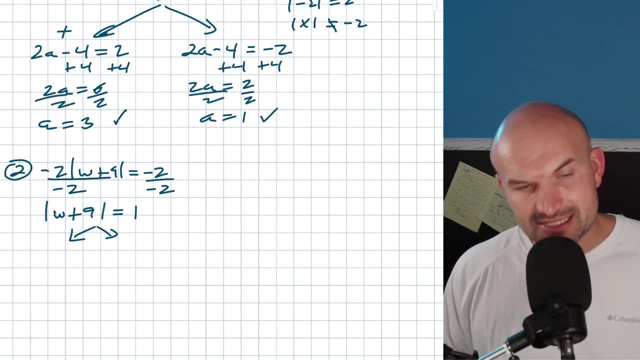 work right, So that's good. So now we can create our two cases. So inside this absolute value can equal to a 1, right. That's what we call the positive case. Or we could say this could also equal a negative 1, right, Because the absolute value of negative 1 is also going to be a 1.. 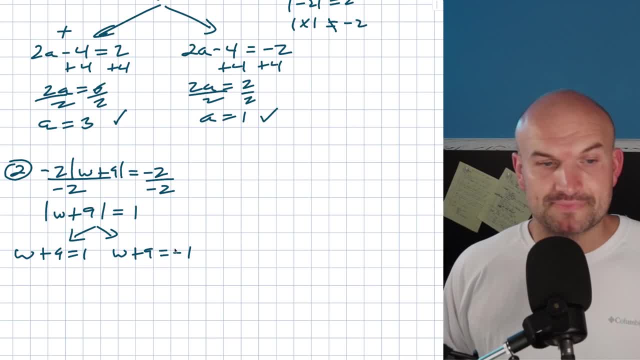 So I could say: a w plus 9 is equal to a negative 1.. Now I can just use my inverse operations, which actually is going to be pretty easy. So I get a w equals a negative 8.. And here I'm going to get a w is equal to subtract a 9.. 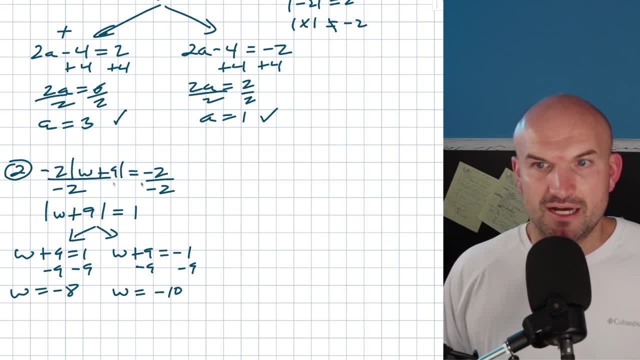 w is going to equal to a negative 10.. And again, let's just do a little bit of mental math. In this case, yeah, just do a little mental math, plugging those values in, And negative 8 plus 9 is going to. 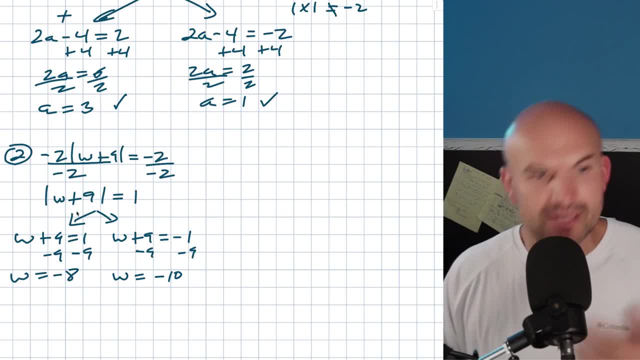 be a: 1.. Absolute value of 1 is 1.. Negative 10 plus 9 is going to be negative 1.. Absolute value of negative: 1.. And you can see that these are both going to work. So what about if we took another? 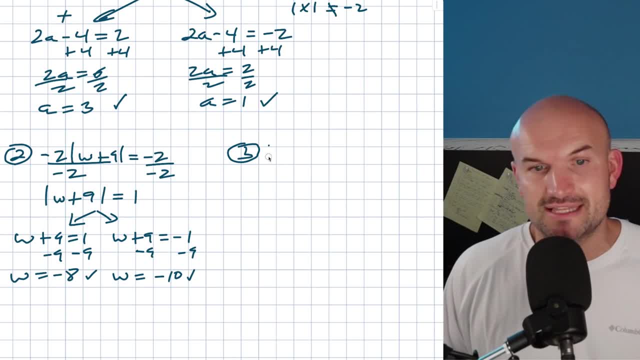 instead of multiplying. what if we had adding or subtracting outside the absolute value? So in this case I'll do: absolute value of b minus 3 minus a, 14 equals to a negative 6.. And again, don't make the mistake right. We see that this is equal to a negative 6.. There are going to be. 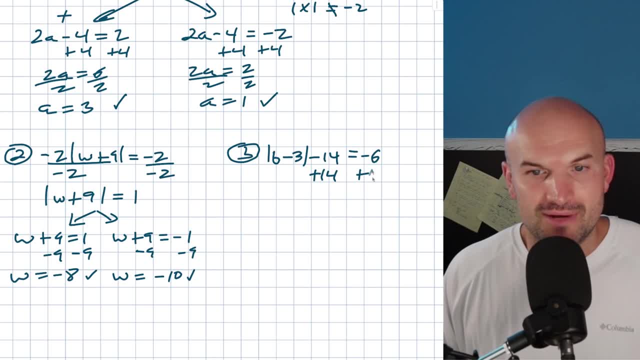 solutions though, in this case, because guess what, When you isolate the absolute value right, you get rid of subtracting the 14. You now have absolute value of b minus 3 is going to equal to a positive 8. So, again, this is going to work Now inside this absolute value. 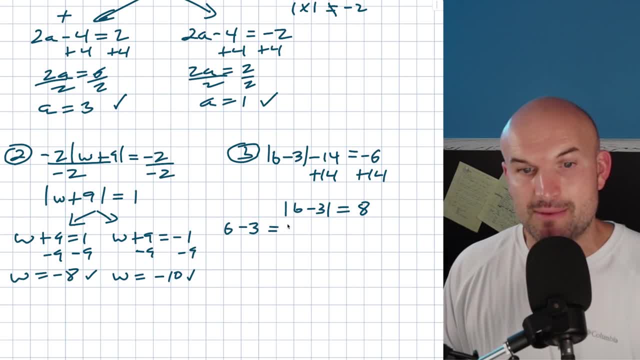 again we have these two cases right. We have b minus 3 could equal to a positive 8. Or we could say: b minus 3 is going to equal to a negative 8. So then again, just use your inverse operations. 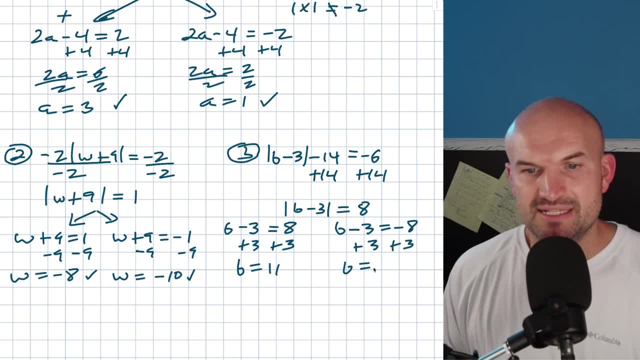 b is equal to 11.. Add a 3 to both sides. b is equal to a negative 5.. And again, I can just go ahead and plug this in Visually, kind of mentally check this to make sure that it's going to work. 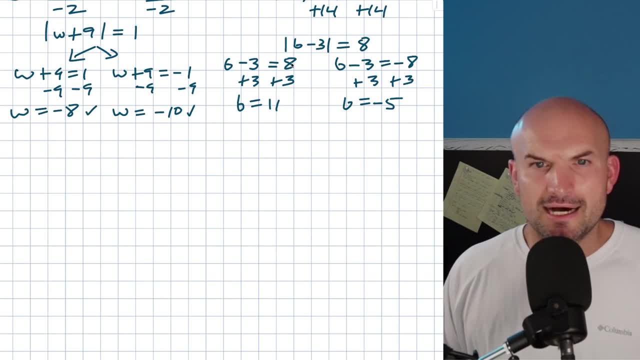 And you can see that indeed it does. So let's go and look at another example Now, what about if we were a radical? So what if I had a 3 times a 4w? minus 1 minus 5 is equal to a 10, okay, So in this, 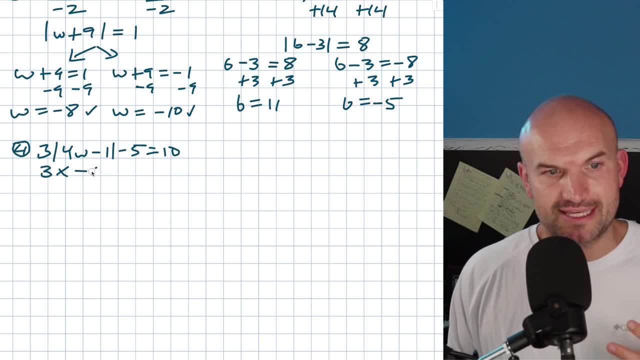 case, what I always like to tell students is like, just kind of like, think of this as like a two-step equation. right, If this was like a two-step equation, what would you do? right? And let me just go and put this, let me actually move this above: Like what would you do on something like? 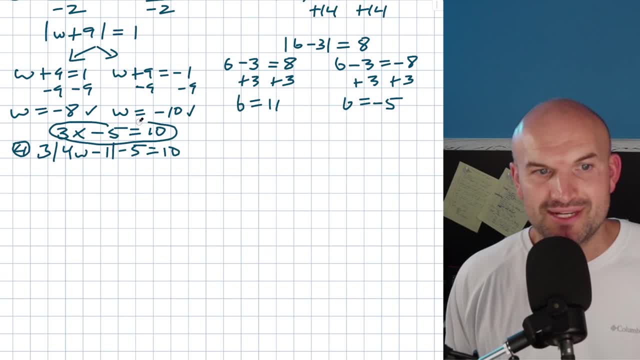 that? Well, hopefully, if you remember, like from your early Algebra 1 days, right? all you're simply going to do is like, add the 5 and then divide by 3, right? So you're going to have a always undo addition and subtraction first, then you undo multiplication and division. 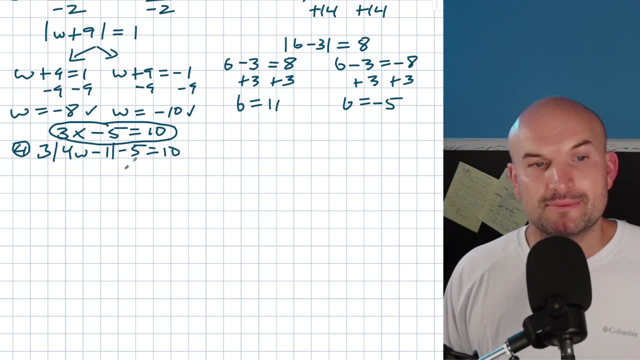 So, by following my reverse order of operations, that's exactly what I'm going to do in this case. I'm going to add a 5 on both sides, And so I get a 3 times a 4w minus 1 is equal to a 15.. Now 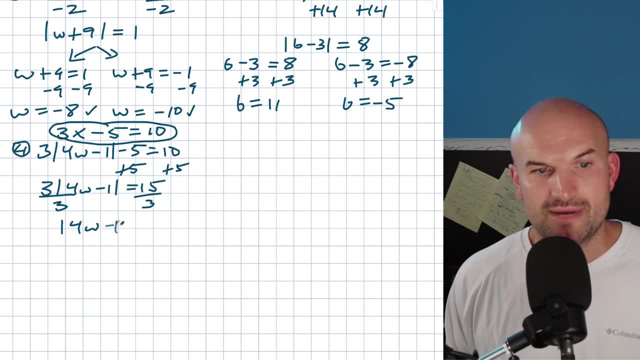 I can just divide by 3 on both sides, get the absolute value of a 4w minus 1 is equal to a 5, right, And now you can see I can create my two cases right. So inside that absolute value, 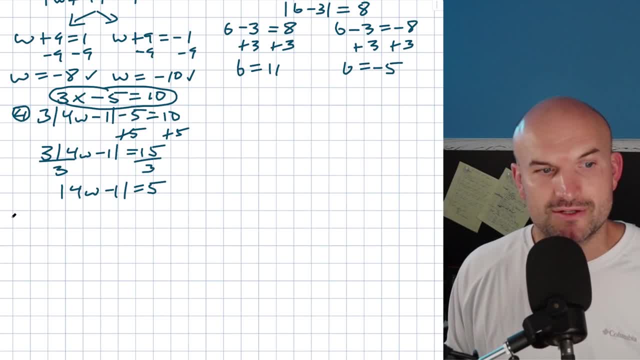 it could be equal to a 5 or it could equal to a negative 5.. So I'm just going to create those two cases So I can say 4w minus 1 equals 5 and a 4w minus 1 is equal to a. 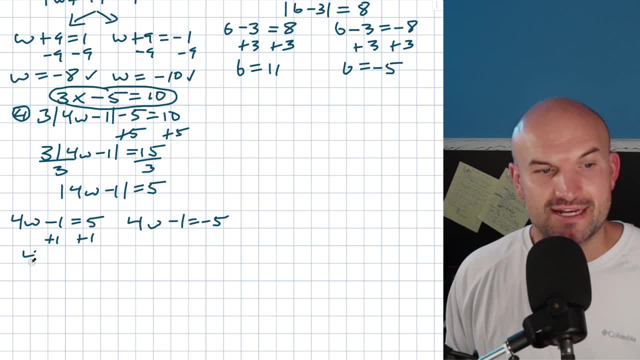 negative 5.. Now I'm just going to use my inverse operations Now again. in this case, what we're going to have is a two-step equation, okay, So when we again we got to undo addition and subtraction first, And then we're going to divide by a 4 so that I can get: w equals a. 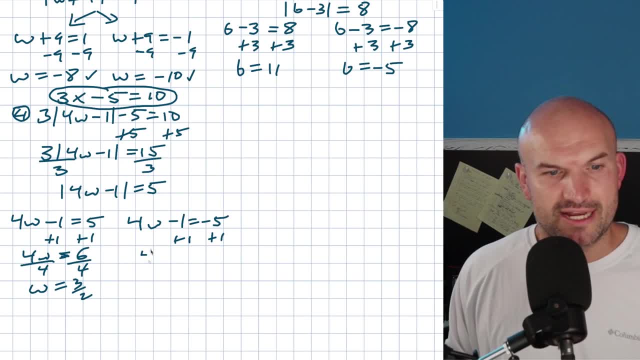 three halves And then this one. I'll add a 1 on both sides and a 4w is equal to a negative 4.. Okay, So divide by 4 on both sides and I can get a w is equal to a negative 1.. Now again. 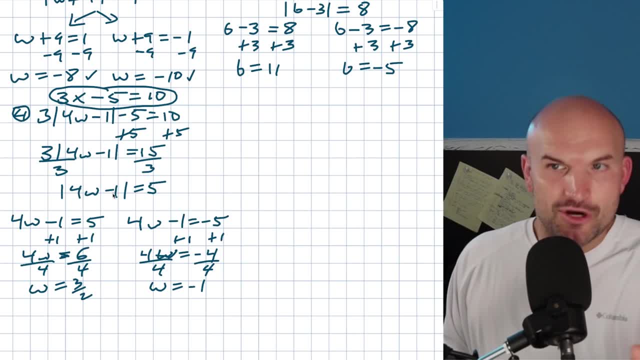 we still want to go ahead and check our work. The nice thing, though, is like I know that as long as that's going to equal negative 5, right, That's going to work. And again, like when you multiply 4 times three halves, that's equal to 2 times. I'm sorry that's going to divide out to a 2 times. 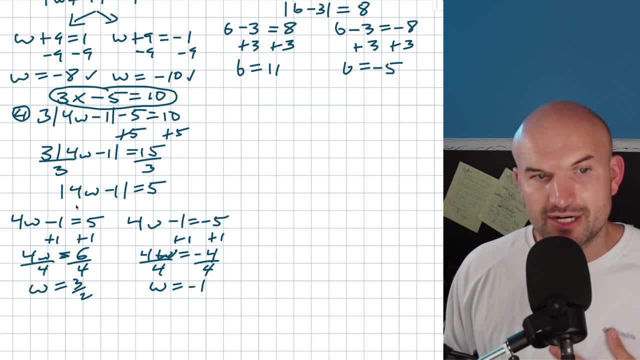 3, which is 6.. 6 minus 1 is going to be 5.. When you plug a negative 1 in here, 4 times negative 1 is negative 4, minus 1 is negative 5. And you can see that these are both going to be negative 5.. 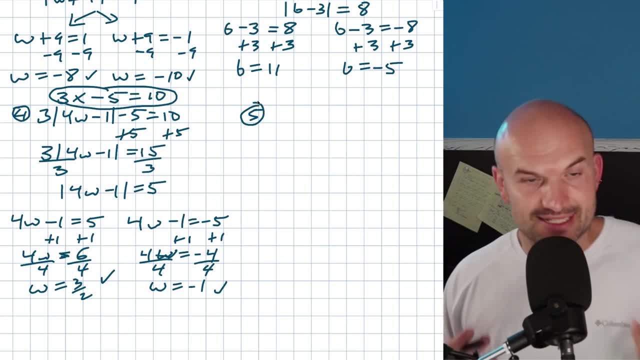 So typically like kind of give you a little bit of hint or a little bit of advice, Whenever your absolute value is just going to be equal to one number. you obviously still want to check your work to make sure that you didn't get an extraneous solution or you didn't do anything wrong, But you 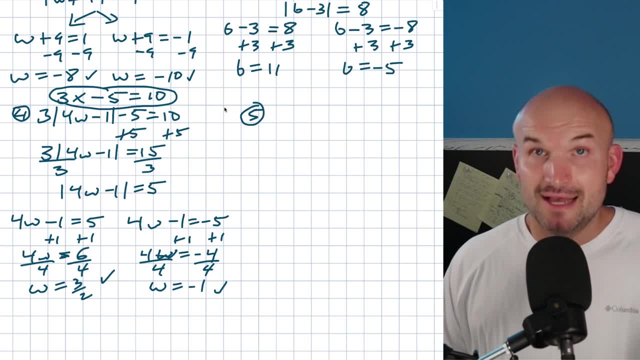 should just be like that. you shouldn't be dealing with any extraneous solutions. However, in the next example, this is where you kind of like your red flags. This is something where you'd be like: uh-oh, I definitely have a very high probability now of having an extraneous solution because 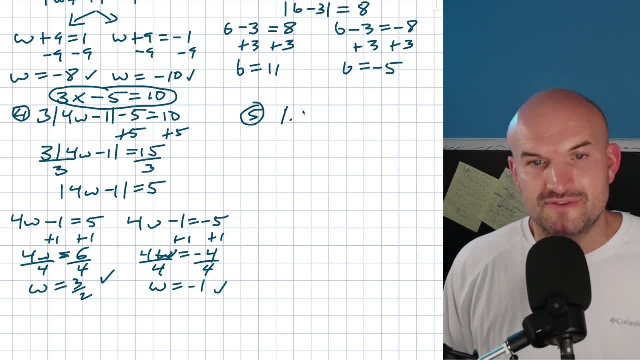 now we just don't have a variable on our solution. So we're going to go ahead and do that. So we're going to go ahead and do that. So we're going to go ahead and do that. So we're going to inside the absolute value. In a problem like this, we're going to have a variable on both sides. 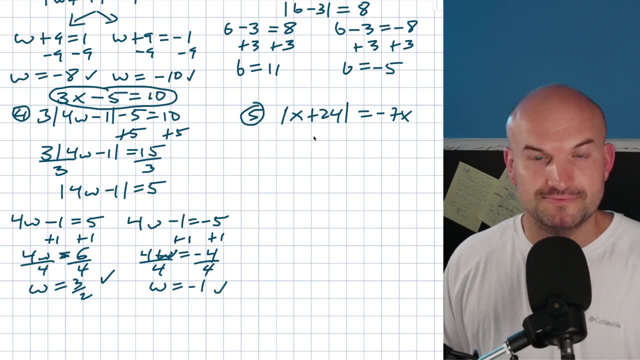 All right. So it's going to be extremely important to also make sure that we check our solutions. So we have the absolute value isolated and you might say, hey, it's equal to a negative. Yeah, but we don't know what X is right. X could be a negative number. Now again. 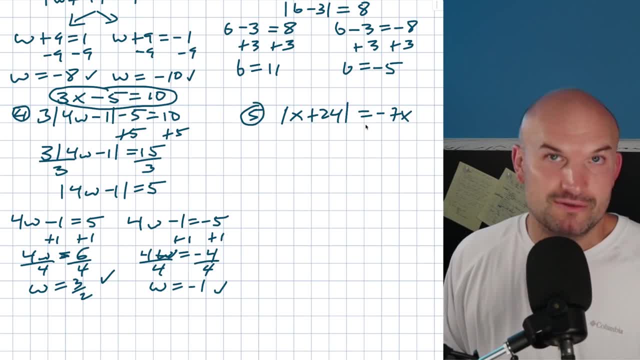 if X is not a negative number, then it would be an extraneous solution, right? So that's something like important to know, So like when we go ahead and solve for our two cases, if we get a positive number right, then positive times, negative is going to make a negative. That's going to be an 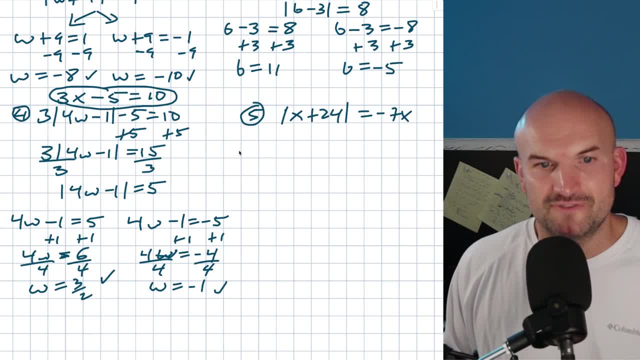 extraneous solution. Let's see what's happening here, All right. So let's go and check to see if we can figure it out. I'll do the first one. X plus 24 is equal to a negative 7X, And maybe run off space, Let me. 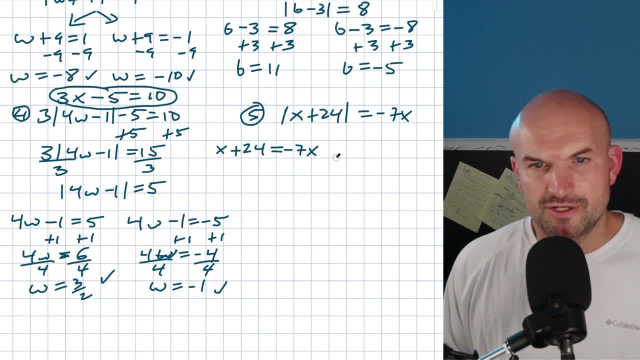 move that over And then I can do a X plus 24 is equal to a positive 7X, right? Because again we need to negate, We need to do the positive as well as the negative version, All right. So if I subtract an X, let's subtract an X. 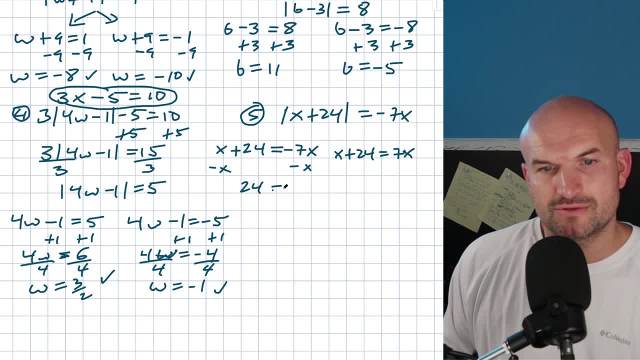 On both sides. So therefore I get a: 24 is equal to a negative 8X Divide by negative 8. Divide by negative 8. X is going to equal to a negative 3.. Okay, And again let's see if that works Like. 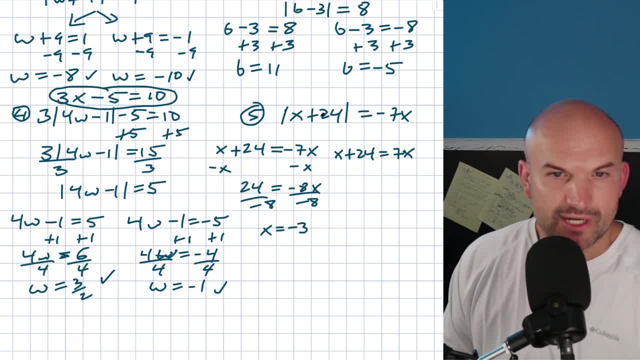 negative 3 plus 24 is going to be 21.. Absolute value of 21 is 21.. Negative 7 times negative 3 is going to be a positive 21.. So that works Now over here, though, if I subtract an X on both. 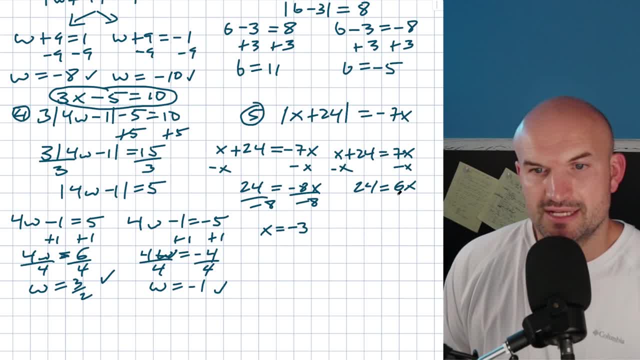 sides I get a. 24 is equal to a 6X right Divide by 6.. Divide by 6. X is now going to equal a 4.. Well, we have a problem here, right? Because if you put a 4 times negative 7, that's going to be a negative 28.. That's going to be an extraneous 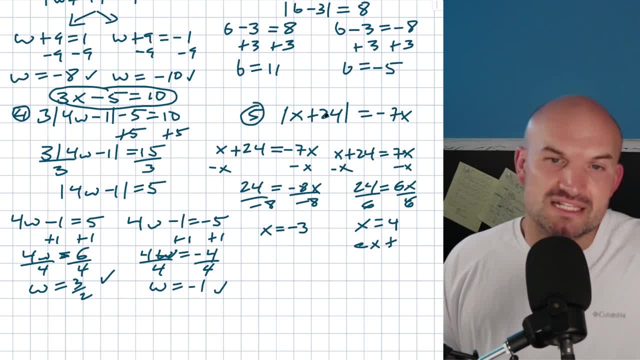 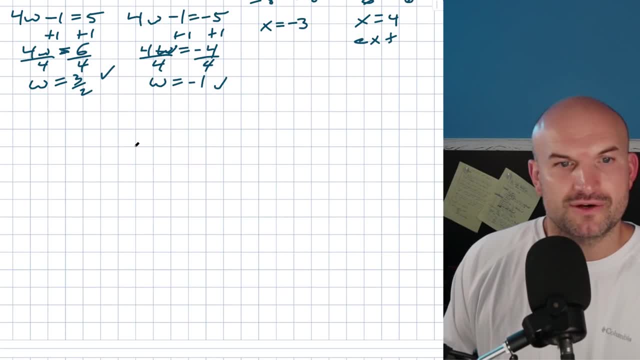 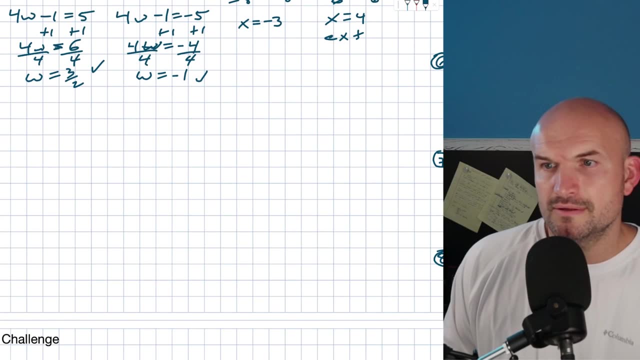 solution. So even though this satisfies this equation, it does not satisfy the original equation. That is why we call that an extraneous solution. All right, Let's go ahead and take a look at. Actually, you know what Let's go and take a look at. Let me see if I can add this in: 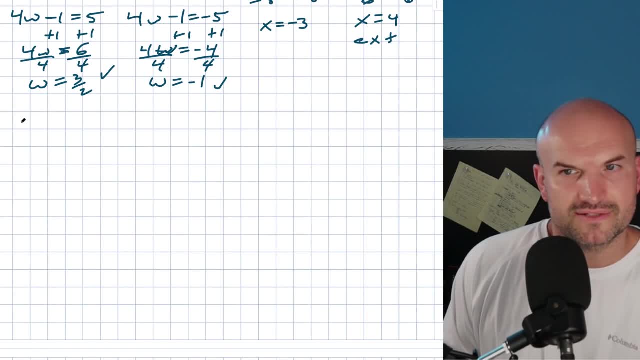 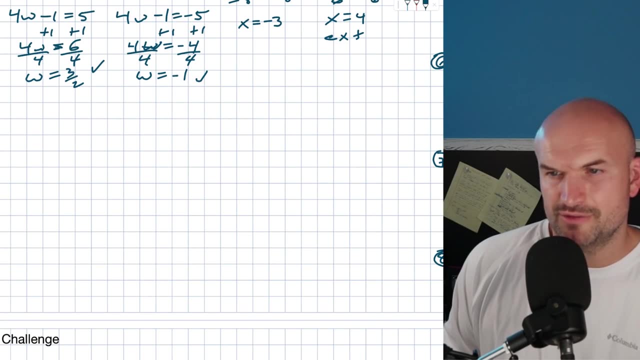 there, All right. So if I go ahead and pick out a- Actually, yeah, let me go and see if I can add a, Add an extra page, just so I have an extra work There you go. OK, I do have extra work, Cool. 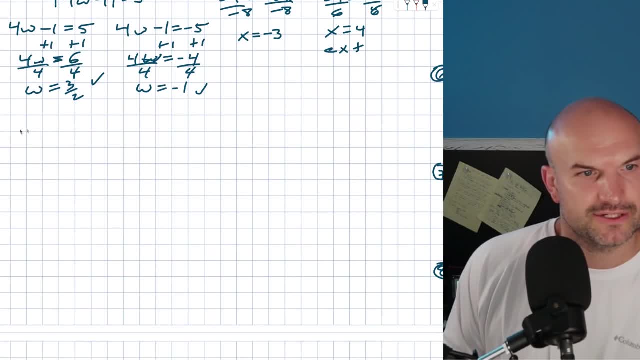 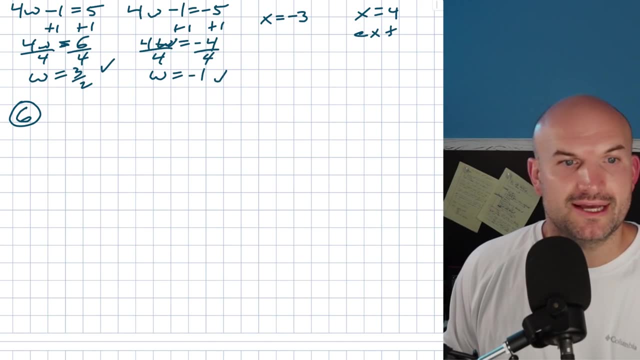 All right. Oh, sorry about that. All right, Let's go ahead and get into 6.. I use a little bit more work on my original equation than I wanted to. All right, So what if we have an equation where we have some operations- not just a operations, also with? 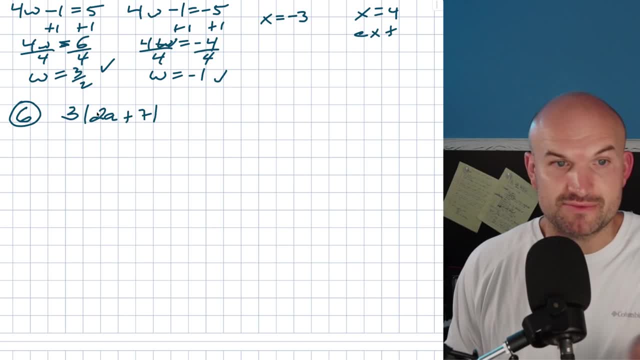 the variable are also with the absolute value, like 2A plus 7, right, So 3 times 2A plus 7.. And then also, not only do we have a variable on the other side, but we also have some numbers. 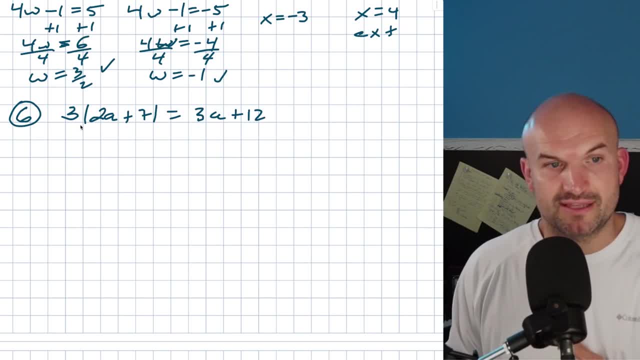 right. So again, the first thing we always want to do, guys- it doesn't matter what's on the right hand side like: isolate, get rid of the any operations being applied to your absolute value, right? So divide by 3 on both sides, and then we have a 2A plus 7 is equal to an A plus 4.. 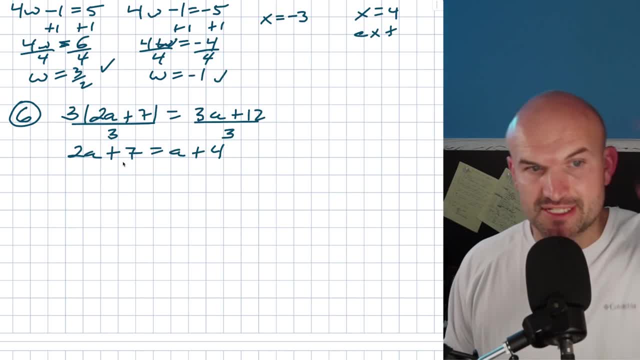 OK, so again now we need to create those two cases Now again. I know sometimes it gets confusing when you're looking at like variables on both sides. But again like the, don't forget the absolute value here. But remember we got to go back to like when we just had a number right. 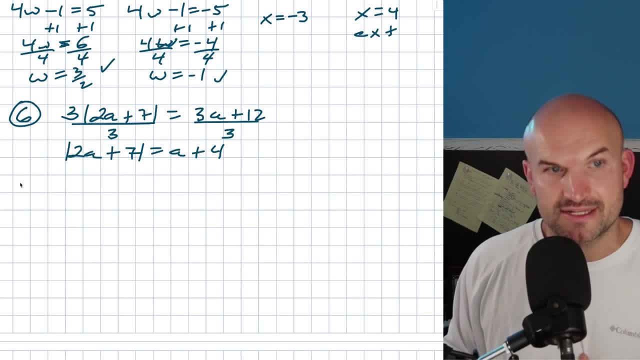 So we're going to go back to like when we just had a number right. So we're going to go back to like when we just had a number like. we have to create that positive case as well as that negative case. So, therefore, the positive case is really just going to be the simplest and easiest. 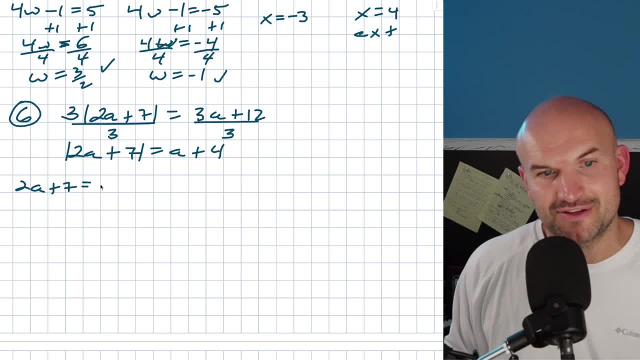 one to straight like: you basically just eliminate the absolute value And now you can have the right hand side exactly as the same. However, for the negate, negated side, what you're going to do is a 2A plus 7 is equal to a negative A plus 4.. So it's really important. 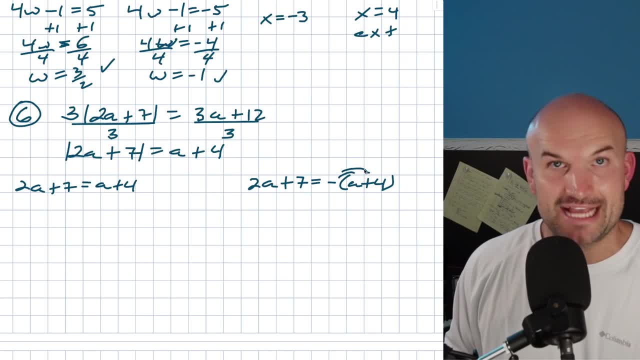 that you kind of understand the use of parentheses here, because you're not just negating the A, you're negating the A plus the 4.. OK, and again, I'm not saying make them negative, I'm saying negate them, right, That's a big difference. So you just make using them to be. 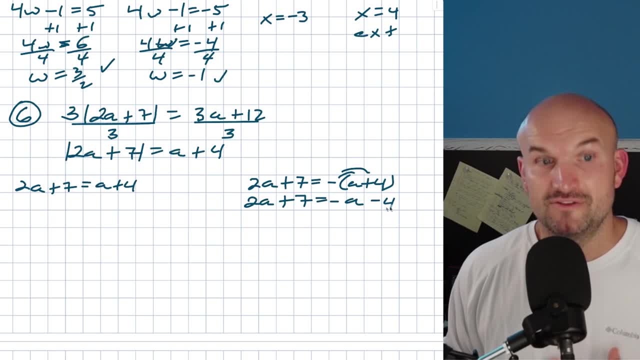 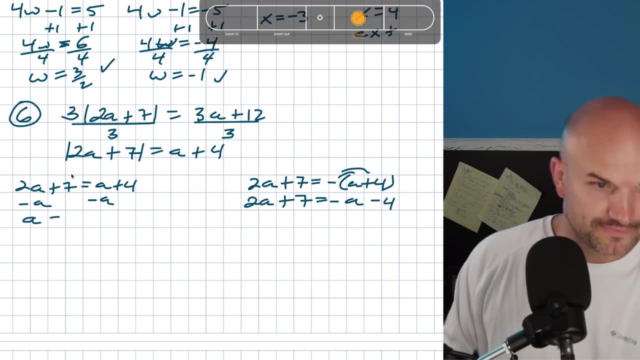 the opposite sign. So therefore it's going to be a negative A minus A 4.. OK, so now we just need to use our inverse operations here. So I will subtract an A on both sides- A plus sorry, A plus 7 is equal to a positive 4- and then subtract a 7, subtract a 7, A is going to equal. 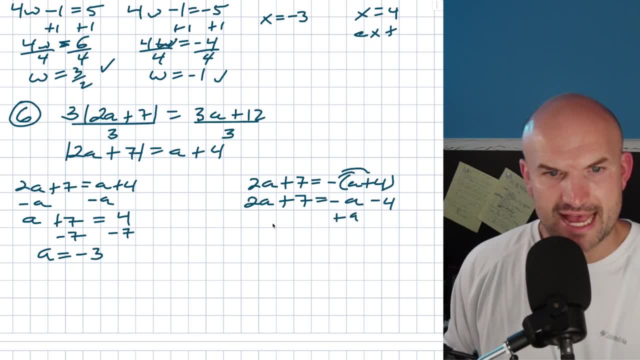 a negative 3.. And then, in this case, what I can do is add an A to both sides, subtract a 7 on both sides and therefore I get a 3A is equal to a negative 11.. OK, so now let's go ahead and divide. 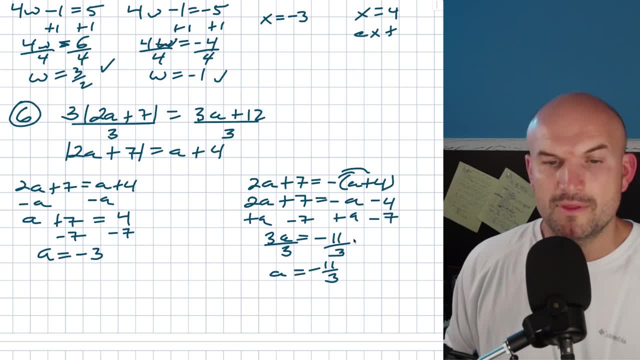 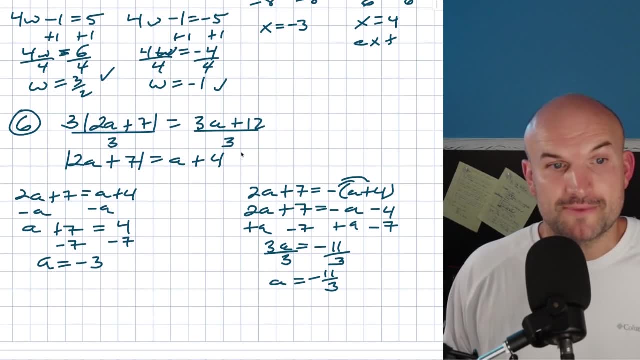 by 3 on both sides and I get A is equal to a negative 11 thirds. OK, so now we need to make to check, though it's like remember last example where we had an extreme solutions, like we got to be able to see. is one of these going to be an extreme solution Now, when I just have this? 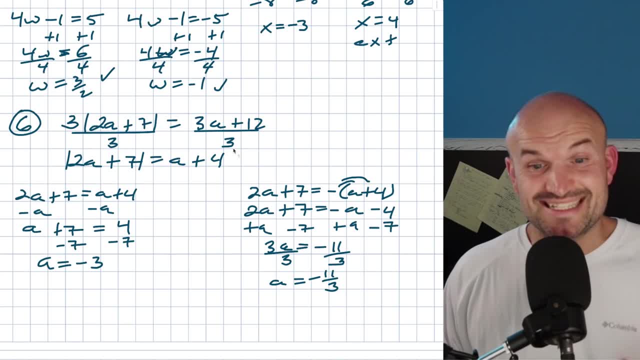 negative 3, like. you can plug them into either the top equation or the bottom equation, It doesn't really matter. OK, so you can plug them into either one, It doesn't matter. Now, what I would prefer to do in this case is, for this example, I'm going to plug it into the bottom equation And then for 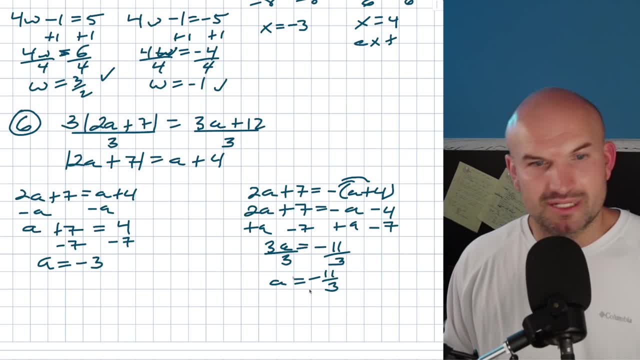 this equation. I'm actually I'm actually going to plug it into the top equation And I'll kind of explain. I'll explain why as I go through it. But in this equation, like, let's just plug in absolute value of 2 times instead of A, it's going to be negative 3, right, Then that's going to be plus 7. 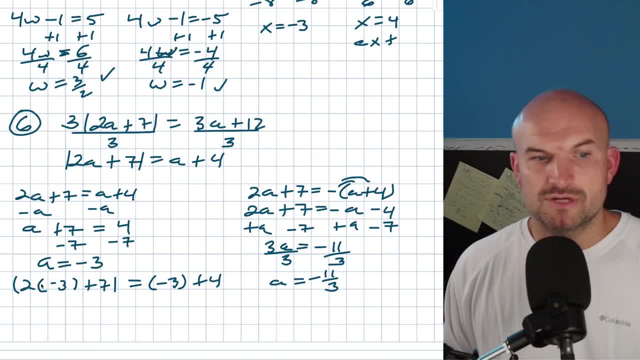 equals a negative 3 plus 4.. OK, so 2 times negative 3 is going to be a negative 6. Negative 6 plus 7 is that's an absolute value. Negative 6 plus 7 is a 1, right. And then I'm going to plug it into the. 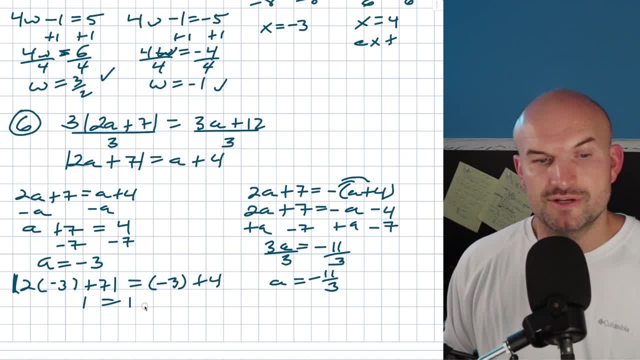 top equation right. Absolute value of 1 is going to be 1.. Negative 3 plus 4 is 1.. So you can see how that one works out. Now the negative 11. third, the reason why I want to plug it into this top. 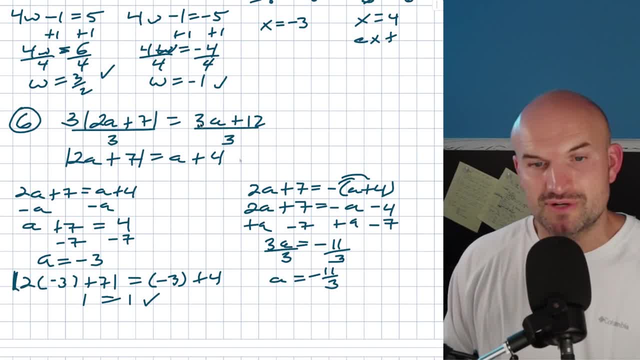 equation is because when I multiply the negative 11 thirds times 3, that's going to get rid of the fraction. right, And in my opinion, like that just makes life so much easier if I can get rid of the fraction, OK, so what I'm going to do is I'm going to say, all right, so I have a 3 times the absolute. 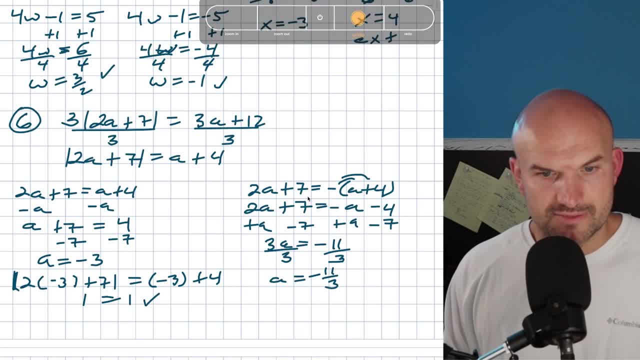 value of. let's actually let's plug it in right up here, So I have the 3 times the absolute value of 2 times a negative 11 thirds plus 7.. Now, that doesn't look like too much fun. Equals a 3 times. 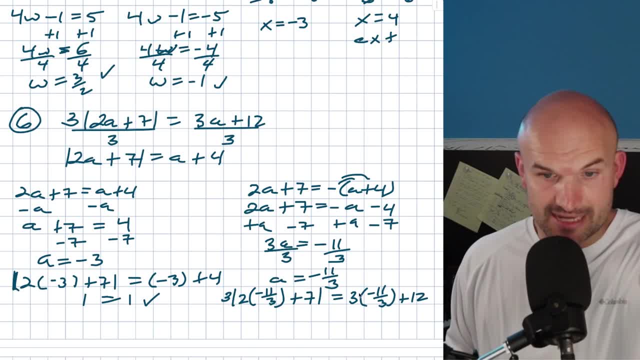 a negative 11 thirds plus a 12.. OK, so again, as I mentioned, like that's technically a 3 over 1, right? So those are going to divide out. So that's equal to a negative 11 plus 12.. OK. 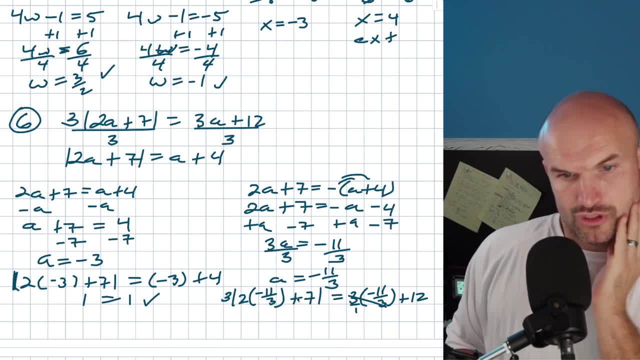 now over here. what we simply needed to be able to do is kind of see: well, how can I rewrite 7 in terms of thirds? So please remember that 7 is the same thing as a 21 over 3, right? So what I? 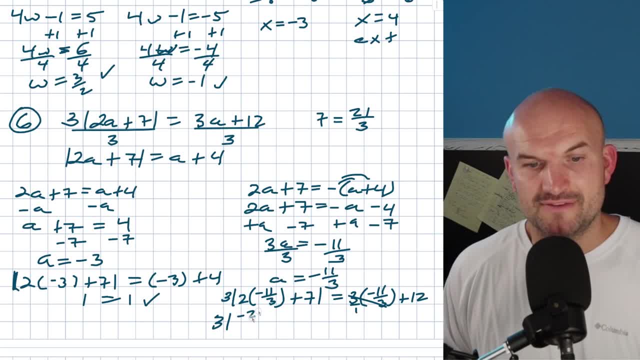 have here now is a 3 times the absolute value of a negative 22 over 3 plus a 21 over 3 equals negative 11 plus 12 is going to be a 1.. Now let's kind of do a little mental math here. Negative 22 over. 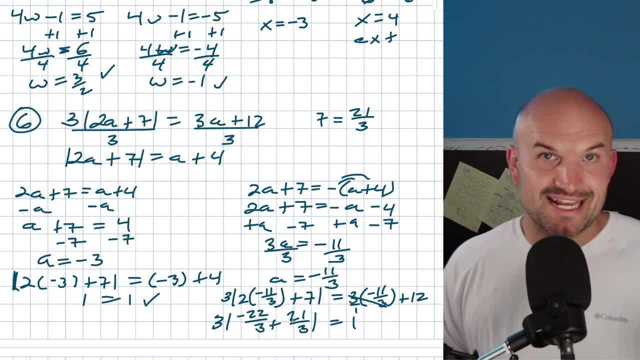 third negative: 22 over 3 plus a 21 over 3 is a negative 1 third. Absolute value of a negative 1 third is 1 third Third times 3 is going to be a 1.. 1 is equal to 1.. You can see that that satisfies Now. 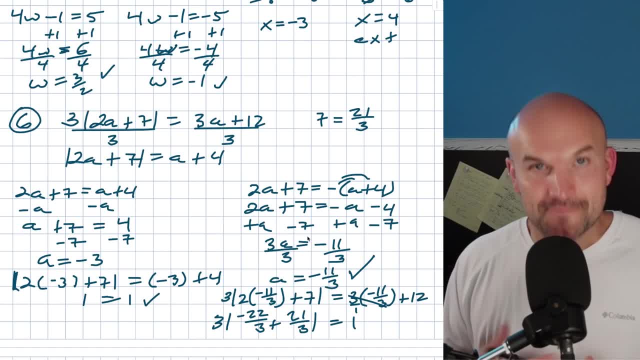 I know at the beginning of this video I said I have eight different examples for you, but I think the next two examples I have are just going to be a little bit redundant. Now, if you need more examples or more help, then go ahead and check out the next example or video. I have for you here: 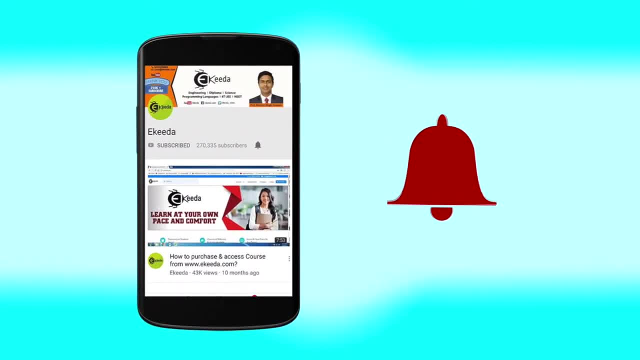 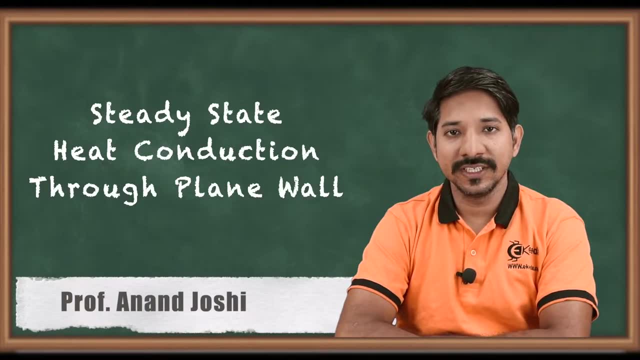 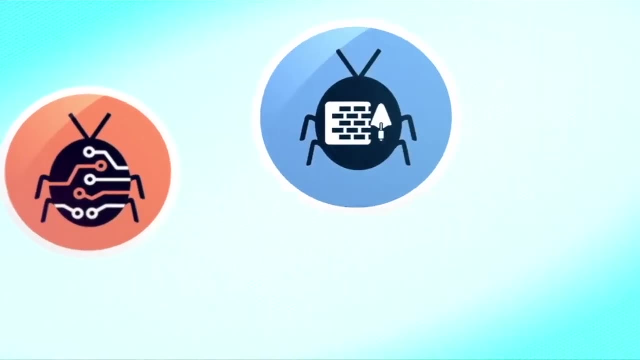 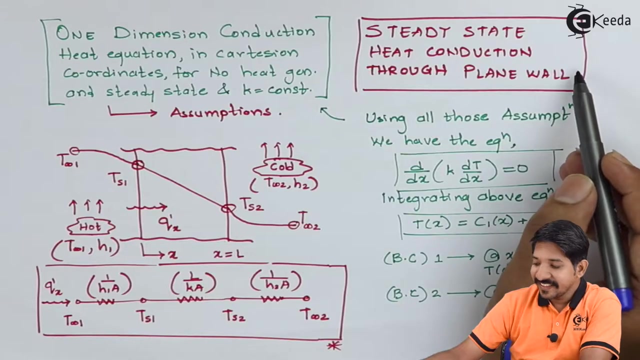 Hello friends, after the derivation of the heat diffusion equation, we need to look into the steady state heat conduction through plane wall. So let us look into that Steady state heat conduction through plane wall. See guys, we have seen previously how